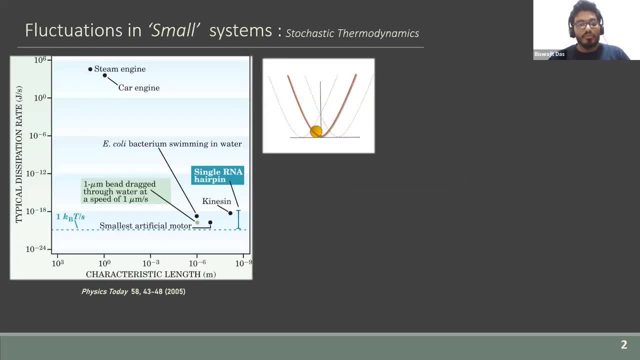 So by now we all know that any microscope processes in microscopic regime, like the position fluctuation of Brownian particle in time dependent trap or any kind of stochastic pump or even the working of kinesin motor, are very driven by thermal fluctuations and stuff like that. 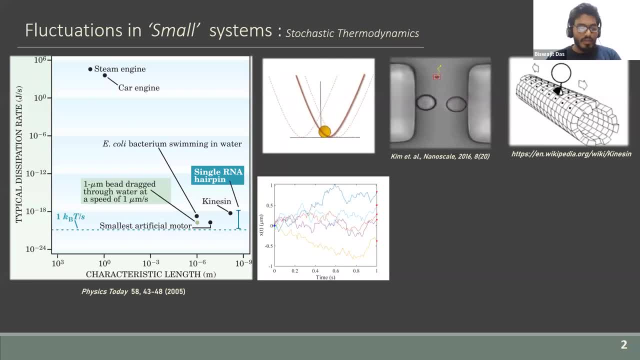 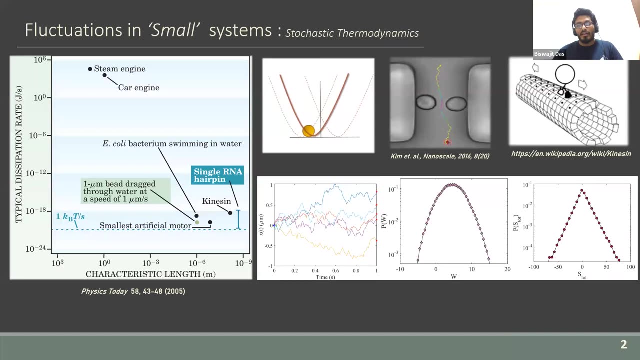 And that's why every time if you realize the system, you will get different, different trajectory. Then if you do any trajectory- dependent thermodynamics- and try to quantify work and entropy, and it like that every quantity will have a distribution and rather than a single value. 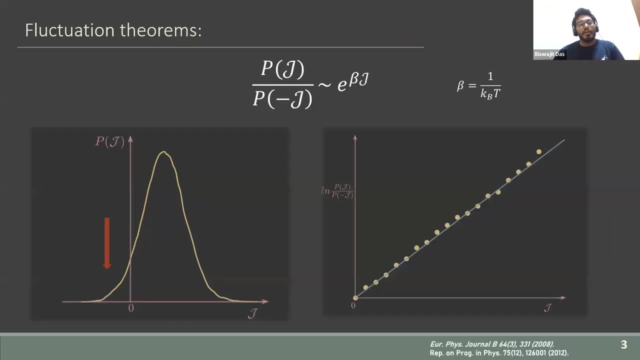 This will have a distribution and there are this fluctuation theorem, which tells us about the probability of the positive fluctuations, and the probability of the negative fluctuations, And they say that The probability of the positive fluctuations are exponentially more So and if you take the log of that you will get basically a straight line curve. depending on the curve, 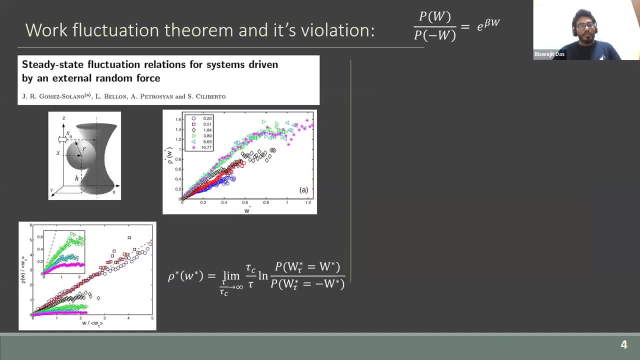 And on this line there is this work fluctuation theorem which is like the relates the positive work fluctuation to the negative work fluctuation. And this fluctuation theorem is very well studied in many different scenarios, Started starting from experiments In colloidal substance, where a particle is trapped in optical tweezers and moved by some kind of external random force. 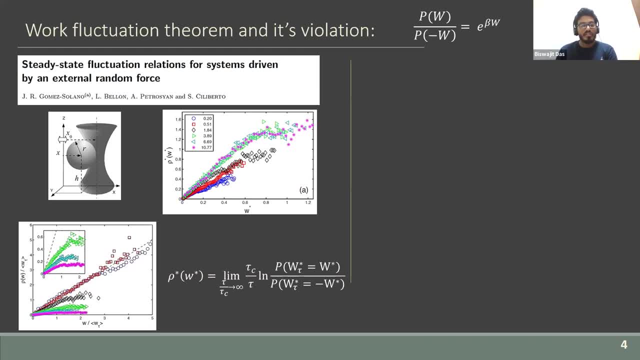 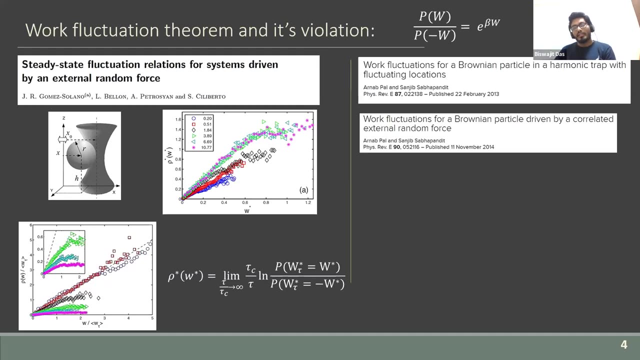 And so that, depending on the strength of the noise, this relation is validated And after, if the strength of the noise is very high, this noise, this, this relation is violated, Then there are other theoretical reasons to talk about this violation And this thing happens. 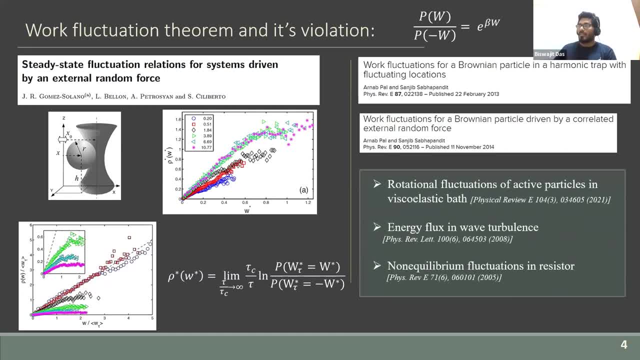 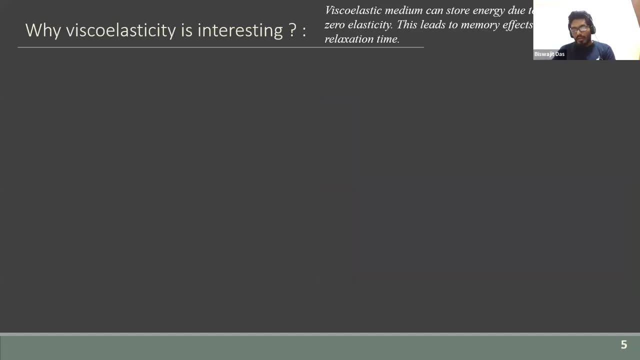 And rather than the colloidal system. many other situations like energy flux in wave turbulence or any electrical register I think there are also these kind of relations- are studied and the violations are well studied. Now we wanted to look into the work fluctuation, as well as the fluctuation of any energetics in a system where the bar is viscoelastic. 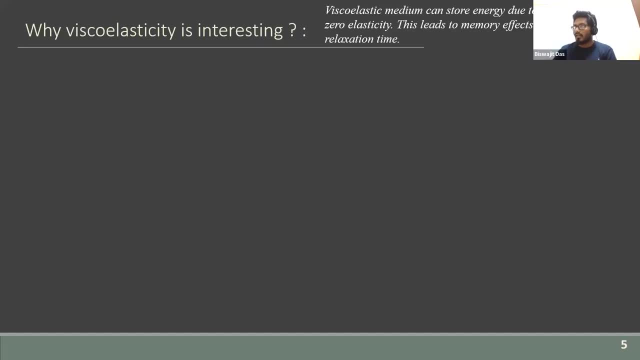 And why viscoelastic? Because Viscoelastic material is like this bath- is not only dissipate energy, but it can some things. It can store energy. that leads to the large relaxation time of the fluid. And in recent times there are these interesting observations, like this enhancement of tremors rate transition and some theoretical estimates of that. 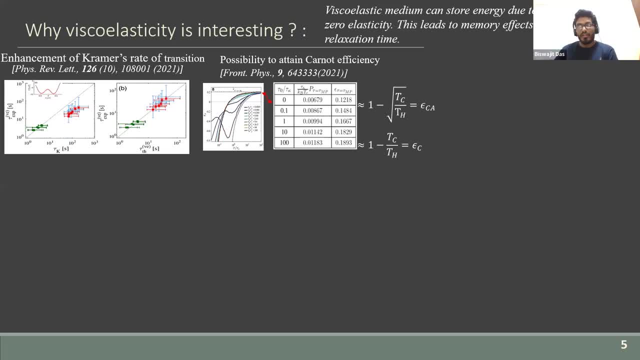 If the bath is considered like viscoelastic, Theoretically the efficiency of Carnot engine Can, possibly efficiency of a heat engine can leads to a Carnot efficiency rather than there are many other thing. If you have a viscoelastic bath and you have active particles, they do so circular motion and they are rotational diffusion and increases. 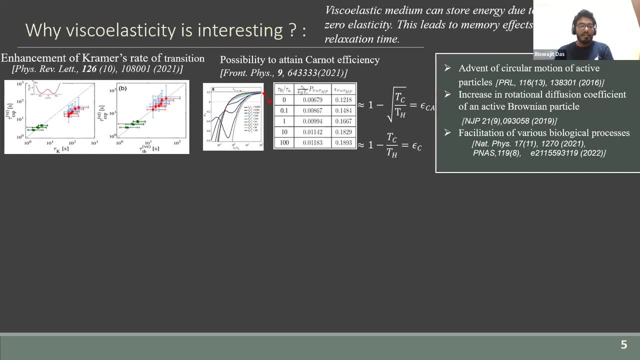 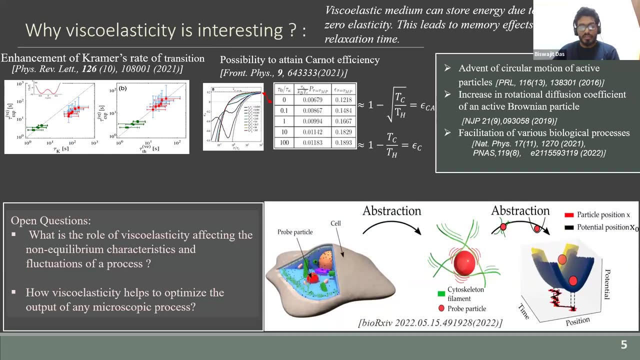 More importantly, there are several papers that shows that in different biological processes are felicitated due to viscoelastic. But still now there are some questions that needs to be answered. That like how this viscoelastic- viscoelasticity affecting the non-equilibrium condition, or how it can optimize the output of such microscopic processes. 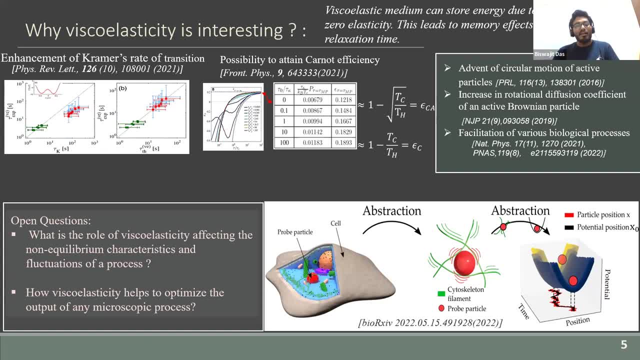 And even you can consider like inside the cell. the medium is viscoelastic And if you put a probe particle there, that will feel the active fluctuations due to the active background inside the cell which you can abstract Like, Like a. 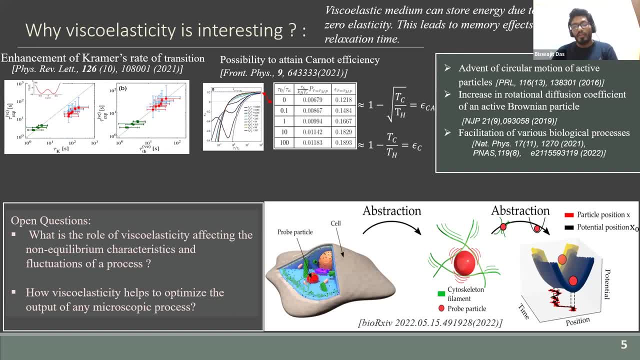 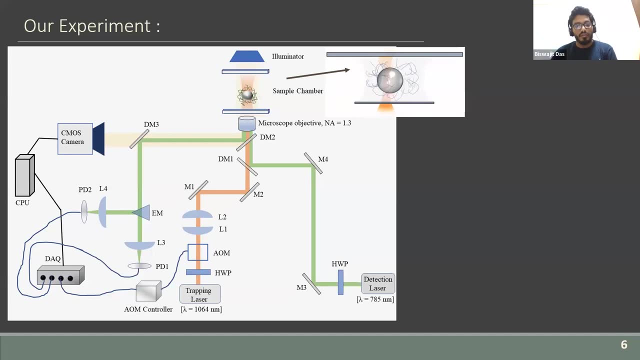 Like a microscopic particle in a Harmonic trap and would strap bodies and it fluctuate. To understand this type of process, We realize our experiment that using optical vision, where we trap a microscopic particle in In, say, polyethylene oxide which is of his coelastic part material. 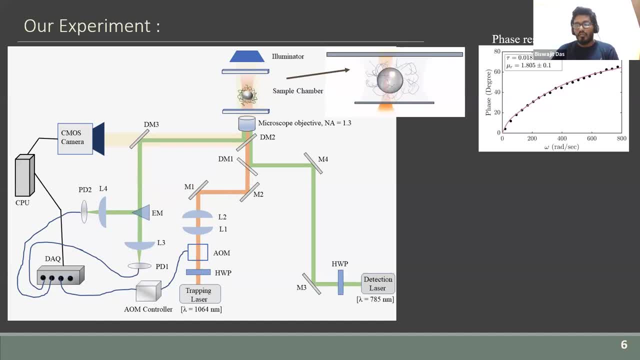 And So then we realize that the time is larger than In his cost material, or something like So, for lessons. and still here We use the material was active on time scale like 0 point 018 a second, And to mimic the activity in the background, what we did, we 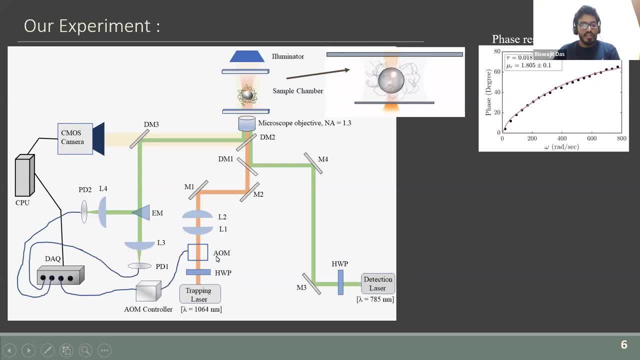 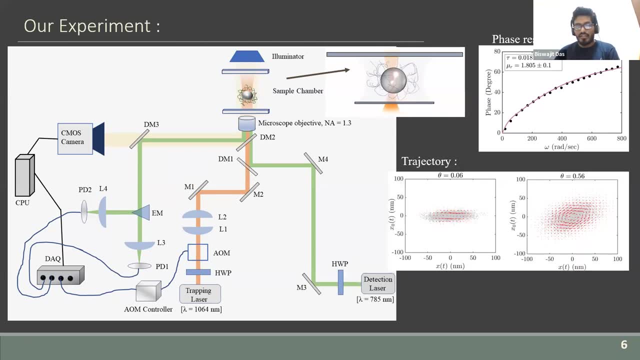 Move the mean position of the trap, Using exponentially correlated noise through these Optic modulator, So that you can see increase the strength of the external noise. the system goes to out of equilibrium and you can see this steady-state current in the background. okay, and to understand this system, 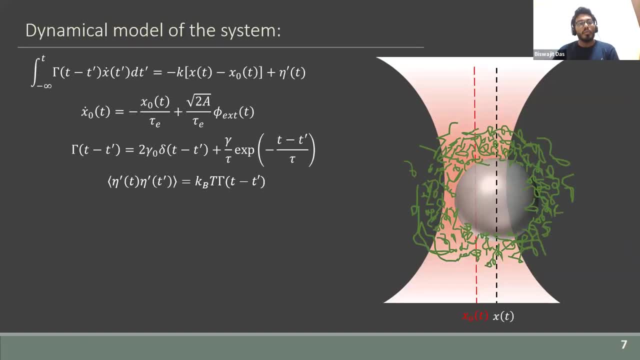 analytically, we write down this, the generalized Langevin equation, with a memory kernel and the mean position of the track is moved like a on-stannulant Begnaud. okay, and this memory kernel, which has a delta correlated term plus a exponential correlated term, this tau. 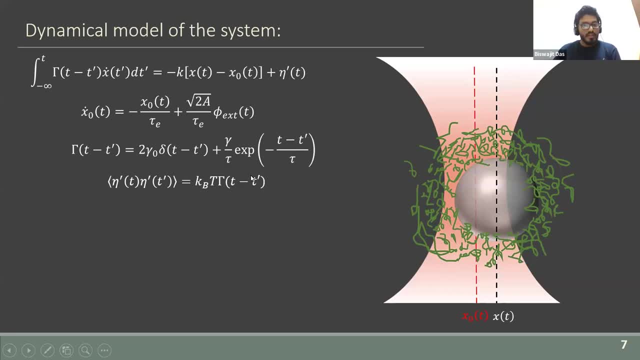 which related to the relaxation time scale of the fluid. okay, so, due to this kind of thing, this Langevin equation is non Markovian and to understand or to solve this thing analytically, to understand the dynamics of this analytically, what we do? we introduce auxiliary variable. 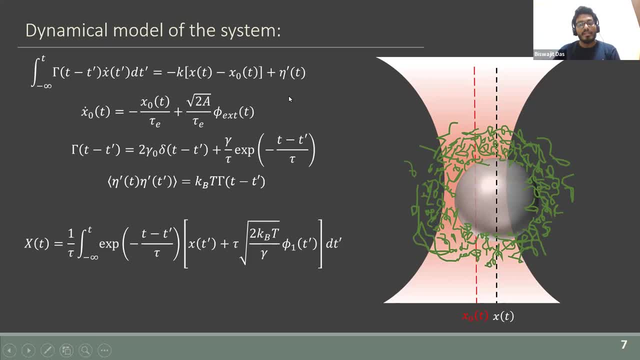 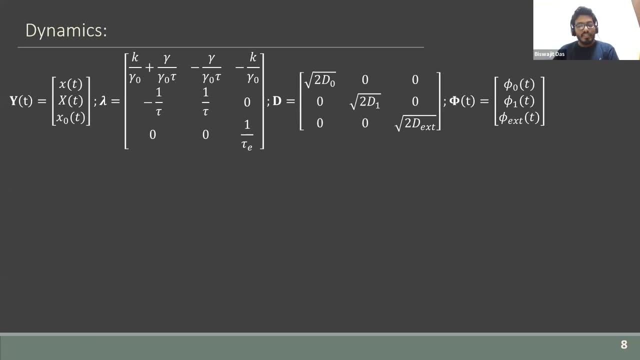 that so that this Non-Markovian system can be written down in a higher order Markovian system so that we can get the steady-state probability distribution of the particle in terms of mean and variance of the fluctuation. So first we look into the variance of the particle. what we first notice, that the variance. 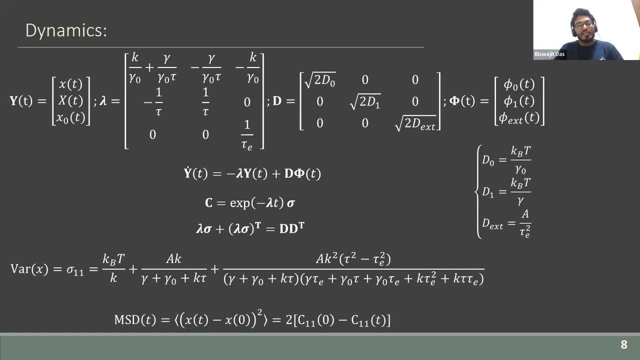 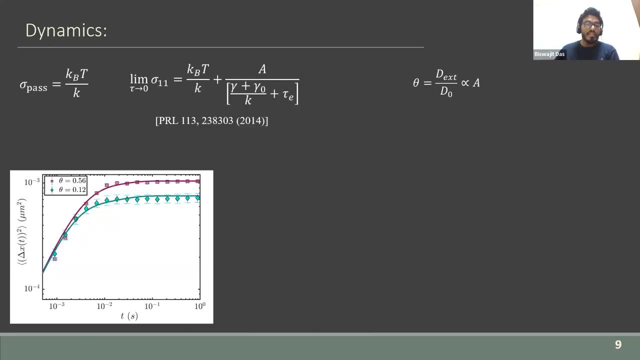 of the particle changes linearly with the strength of the noise, which is here a, and also we look into that In from the mean square displacement and as we see that mean square displacement is increases for a higher noise state, as expected, it increases in the higher mass. then what we, what we notice? 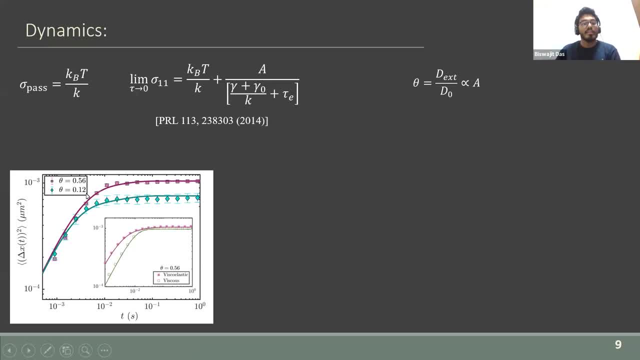 that for a certain fixed noise strength which is determined by this parameter, theta, that we saw that for a viscous case, for a viscoelastic case, the variance, or you can say the effective temperature of the It increases, then the viscous bar, and this nature is here also in the in the steady-state. 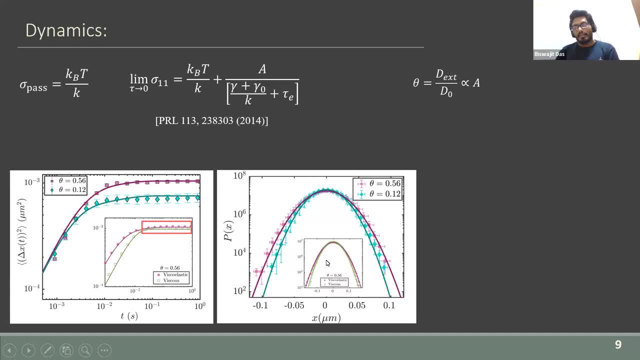 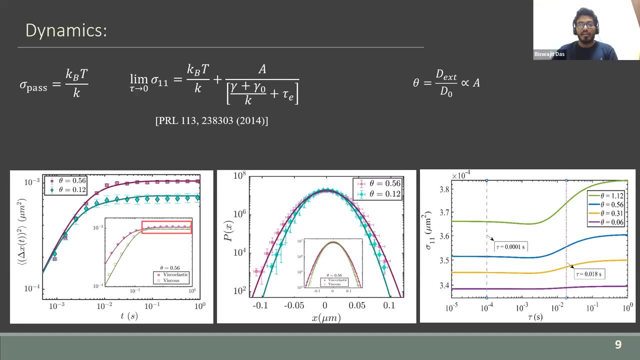 probability distribution too. Also we notice that is variance of the position, fluctuation of the particle and does not change monotonically with the relaxation time of the fluid, but it changes non-monotonic fashion and after some point it does saturate. does not mean if you increase the relaxation fluid. 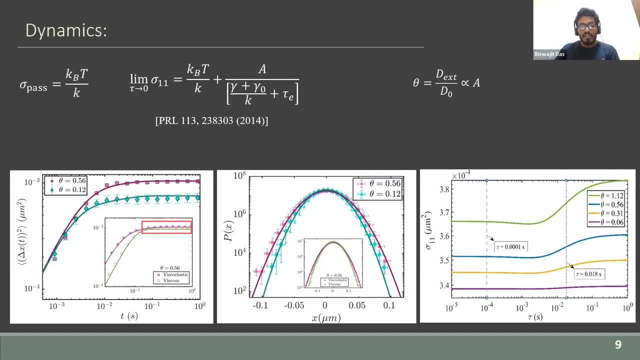 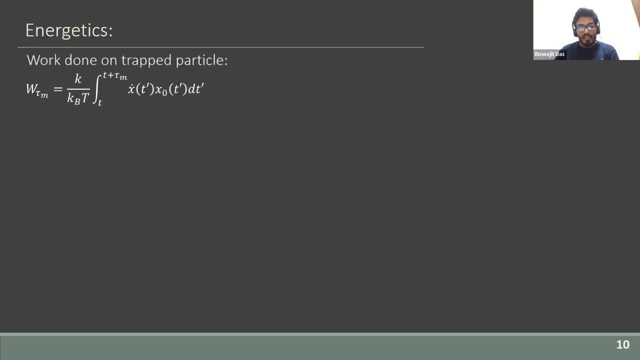 the Sigma Variance does not keep on increasing, but it saturate at some point. next we look into the Energetic. first we look into the work done on the trapped particle and which is defined like that. this is just a force times, the displacement and force time velocity over dt. so this is 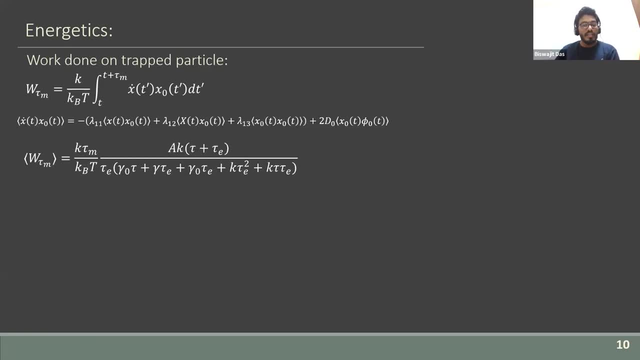 this and then we able to calculate the mean of the work done. and we find out that the rate of mean work done Each one of the Variance does not keep on increasing but is saturated at some point, Each more in case of a viscous elastic bar than the viscous bar. okay, and here also with 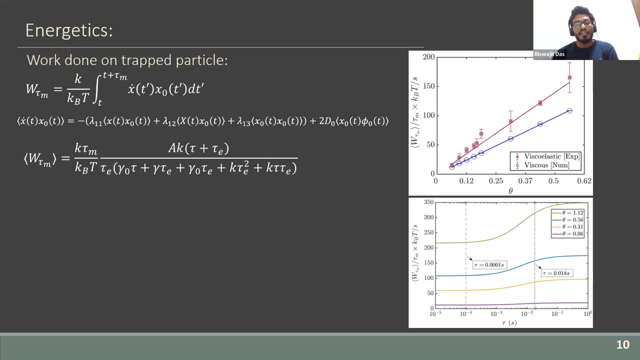 relaxation timescale of the fluid we get, similar nature, and that we saw in case of a, in case of a viscous, elastic, okay. so then what we saw? that the entropy production rate of the system Is found to be exactly equal to the Work done on. 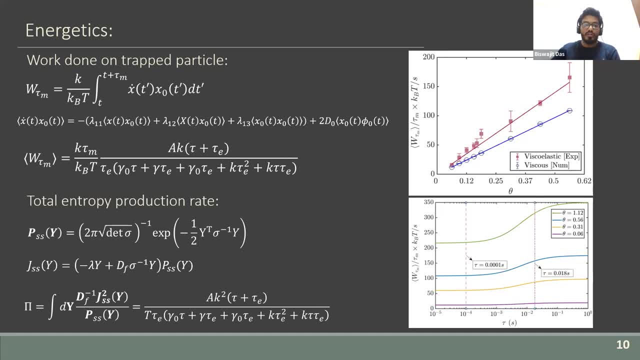 Mean work done on The trap particle. that's because if you look into the entry production current there is only the time extensive part. is the input work done. that is the only extensive part. so the mean of this thing is equal and we we kind of expected that the mean rate of 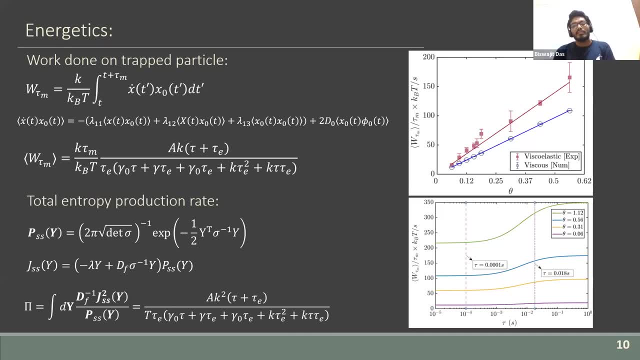 entropy, production or as well as the work done. it increases in case of viscous elastic bar because In viscous elastic bar There are the Increase of Interaction Of the Particle with the Bar due to A different kind of polymer present in the viscous elastic bar and 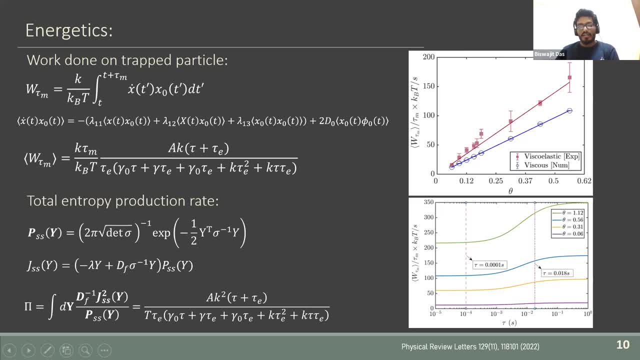 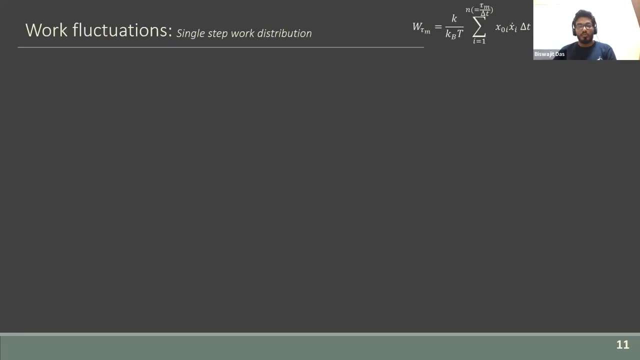 And we know from Recent literature that we know the interaction increases. the entry products are there. so that's why in this holistic bar entropy increase or the work done on the trap particle is increased. then we look into the Fluctuation. so to understand the fluctuation of the thing, first we look at the single step. 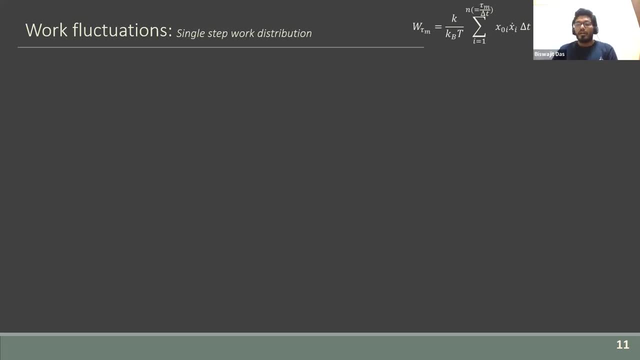 work distribution. So Here we To theoretically understand that what we do. we take care of the fact that this X0, which is the mean position of the particle, and X dot are two Gaussian random variable which are cross correlated, and we so then the single step work fluctuation can be explained. 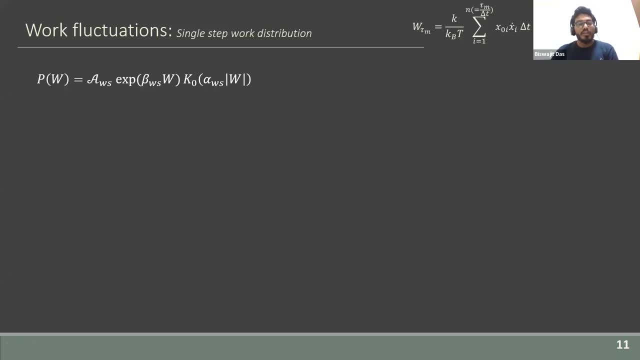 can be expressed in terms of a skewed, This Zeroth order basal function, modified basal function, Where this beta WS and alpha WS term can be expressed in terms of the mean and variance of the Particle. And then what Of the work? 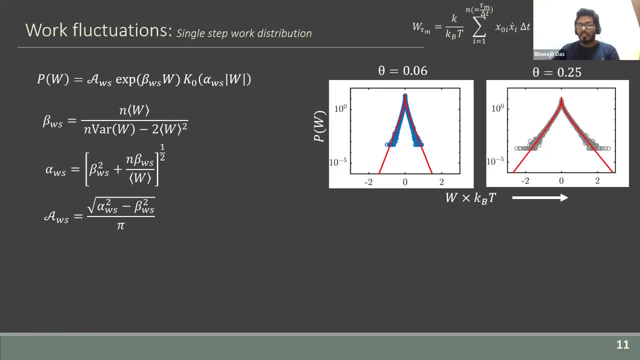 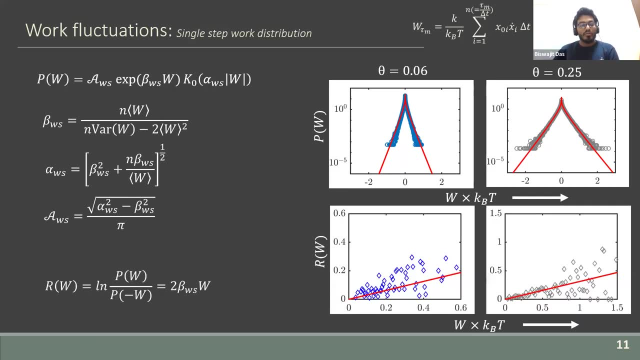 So we saw that Our Theoretical prediction is matches well with the Experimental data from where we calculated the Single time of them. and Also, if we look at the The Work fluctuation theorem, It also matches with the theoretical facts. 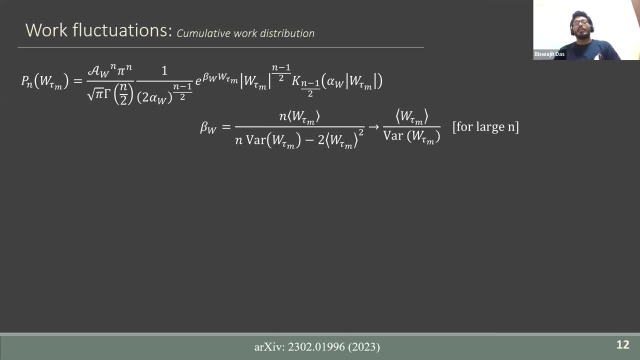 Then we Look into the cumulative work distribution thing. But For the cumulative thing the work Series is Already correlated, right? so We kind of Approximated the correlations of that, Approximately the correlation in the mean and variance of the particle. 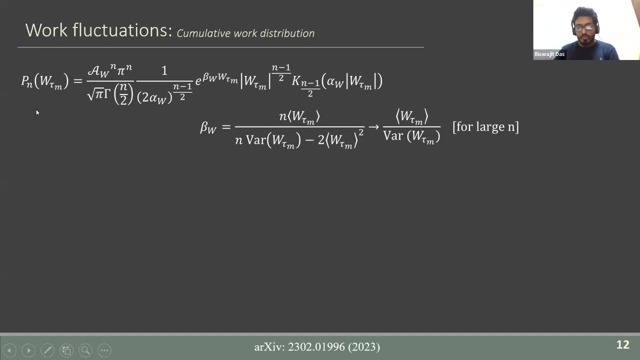 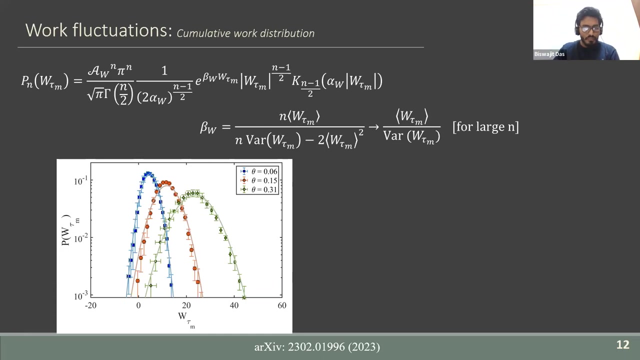 And we Kind of approximate This, This, The Fluctuation in terms of the modified Basal function, and such that It matches well with our Experimental, Experimental Measured Input And what we Notice, That 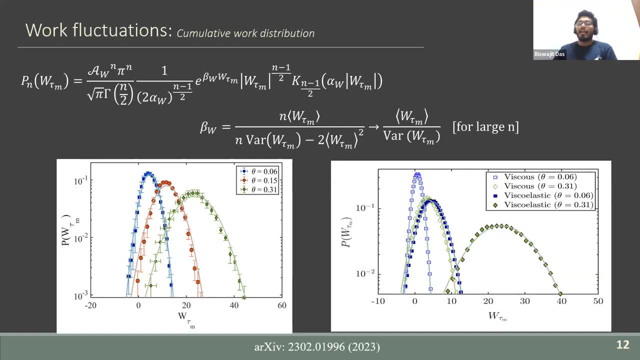 At Long Time. The cumulative The In the Viscoelastic Cases For a Certain Strength Of the Noise. The Negative Work: The Probability Of Getting Negative Work Diminished. 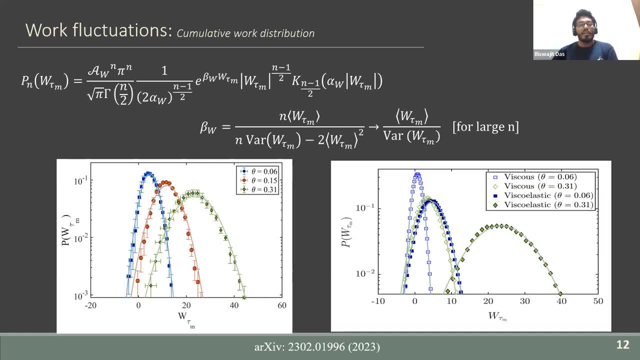 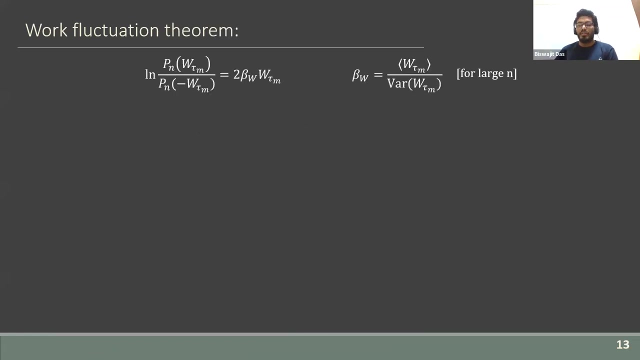 Compared To The general Method, Like The Last Deviation Of Probability Of The Path Probability Measure, Where Also You Can Get This Type Of Long Time. 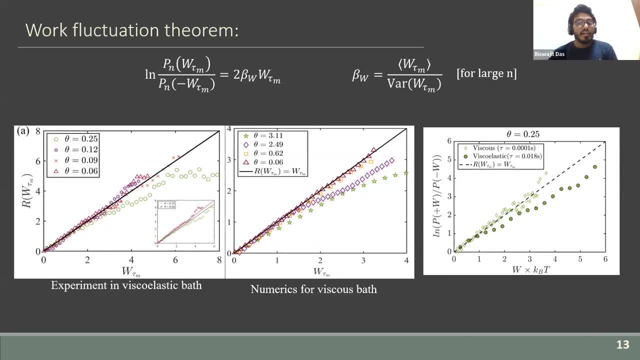 Behavior In A More General Theorem For A Viscoelastic Case Is Violated With A Lower Noise Strength Than The Viscous Case, So For 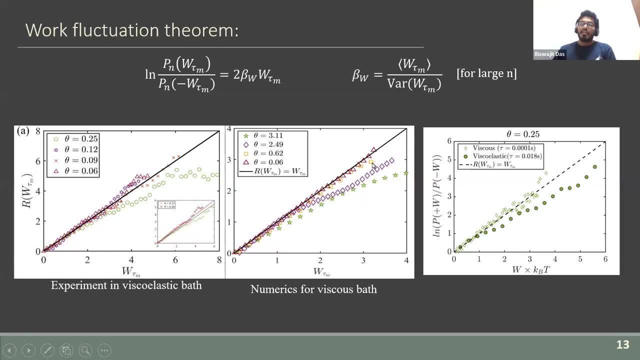 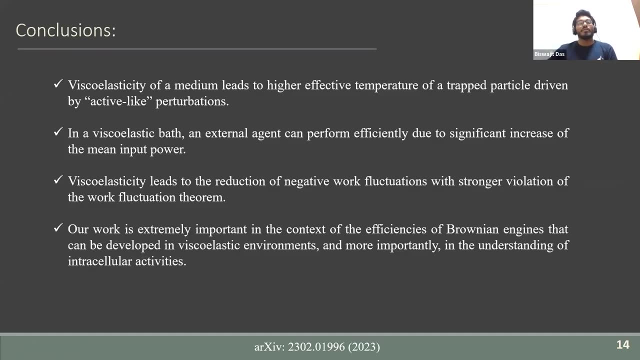 If We Notice That This Even The In A Viscous Case, Even For The Very Lower Noise. So As You Hold What, We Notice That 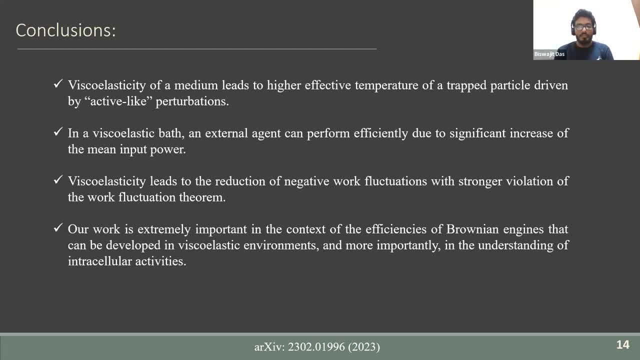 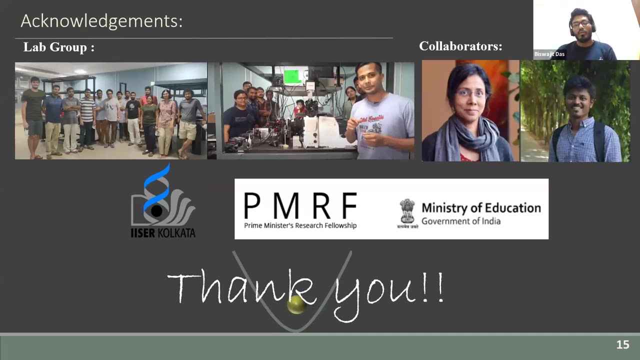 We Thought Viscoelasticity Of A Medium Increases The Input Work Done On The Trap Particle And I Like To Thank My Collaborator, Professor Supriya. 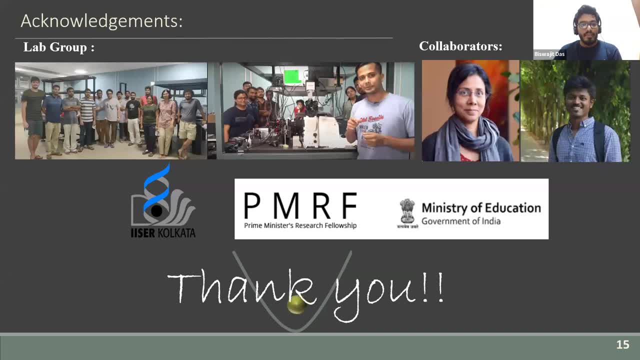 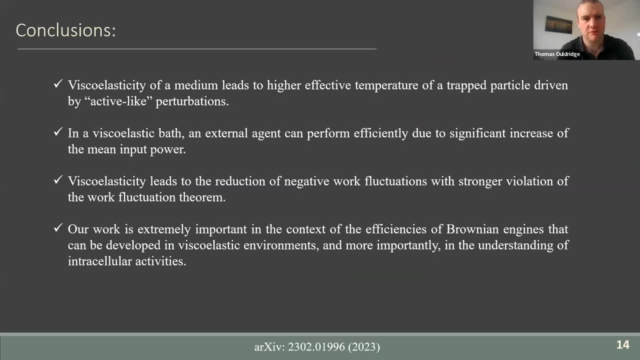 Krishnamurti Srikant From Stanford. So I Would Like To Thank My Funding And Thank You For This. Any Question? Thank You So So. 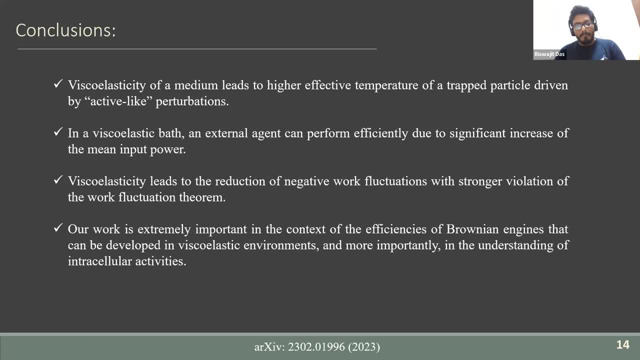 This Is Going Up In The Viscoelastic Case. Yes, Yes, My, My Sort of Intuition, For When You Get Entropy Production From A System. 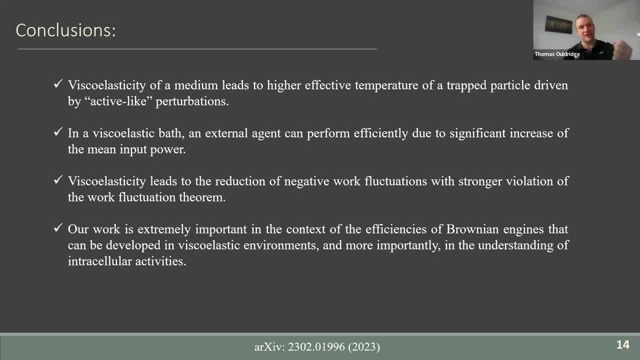 That You're Jiggling Right, Because Then It's Like You're Doing Quasi Static Jiggling, But You Get High Entropy Production When The 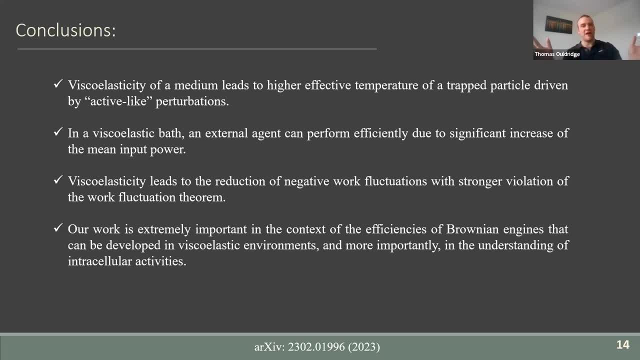 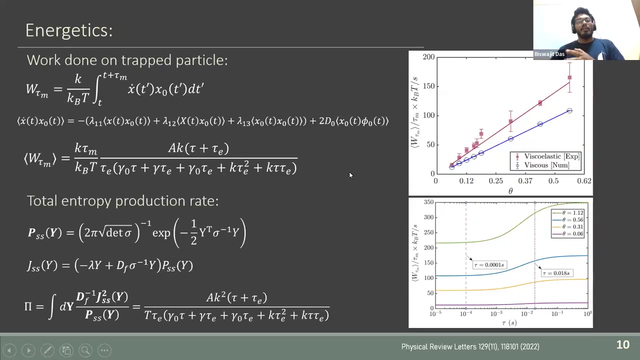 System Is Responding To Your Perturbation But Not Keeping Up With It. Yes, Kind Of, But We Think That. So There Is This Thing. So